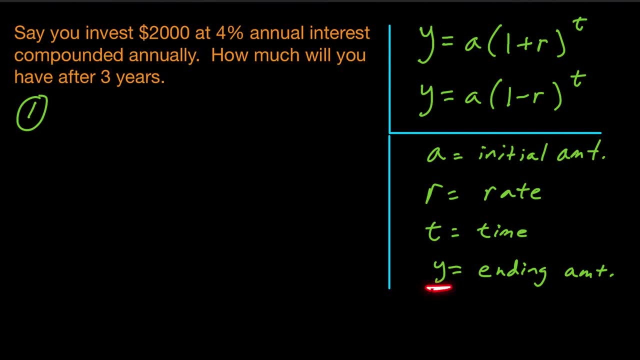 on how the problem is set up. i'll show you some examples and then y is the ending amount. so what you end up with after t years or t months or t days, depending on the problem. so this whole base here, this one plus r that represents the uh growth factor, and this one minus r here represents 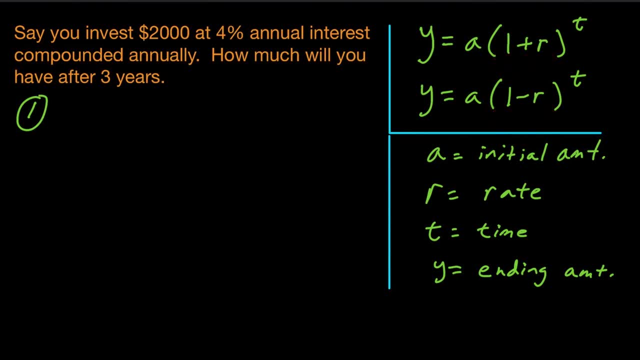 the decay factor. so that base is going to tell you if it's bigger than one that's going to be growth, and if it's between zero and one it's going to be a decay. and then you just have to to ask yourself sometimes you know how much more than one is it That's going to the amount more? 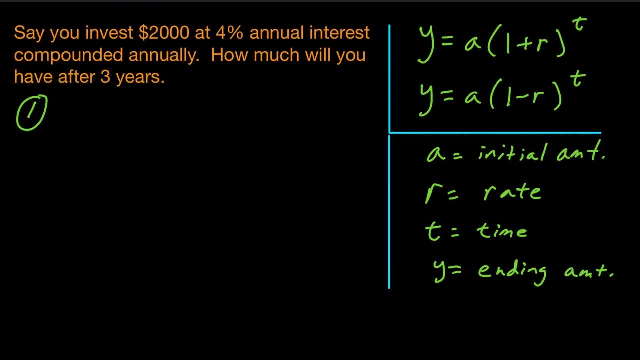 than one is going to be your rate of growth and the less than one that's going to be the amount that's going to be how much less than one it is is going to be how much it's going to be decaying by. So we'll look at some examples. So the first example we're looking at here is, say you invest. 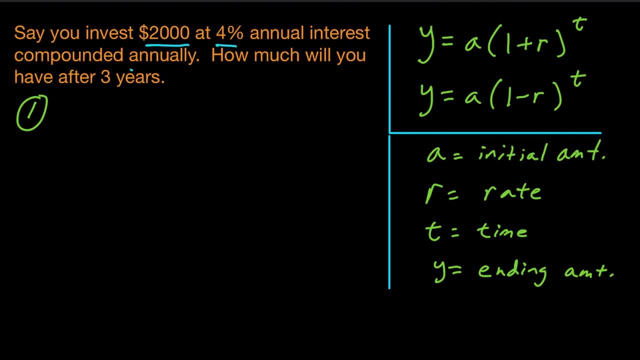 $2,000 at 4% annual interest and it's compounded annually. so just once per year, how much will you have after three years? So because this is a growth problem, we're going to use that top equation: y equals a times one plus r to the t. Our starting amount a is 2,000 and our rate of 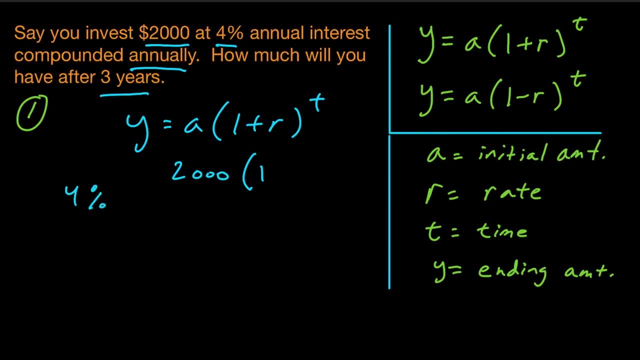 growth is 4%. Now, remember 4%. to convert that to a decimal, you move the decimal two places to the left, so that's going to end up being 0.04, and the time? that's, in this case, three years. So if we 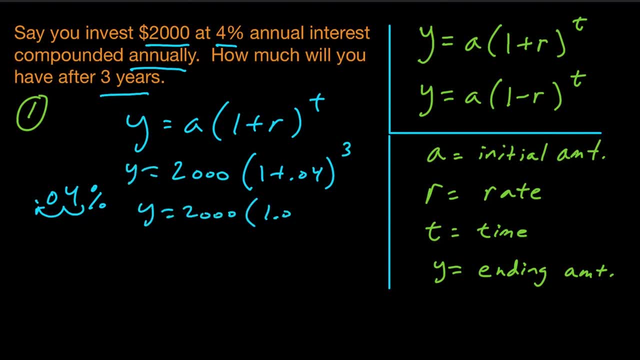 simplify a little bit. we get: y equals 2,000, 1.04 to the third. Notice: this base here is greater than one, which means that this is going to be an exponential growth function. It's going to grow, it's going to get larger and larger. 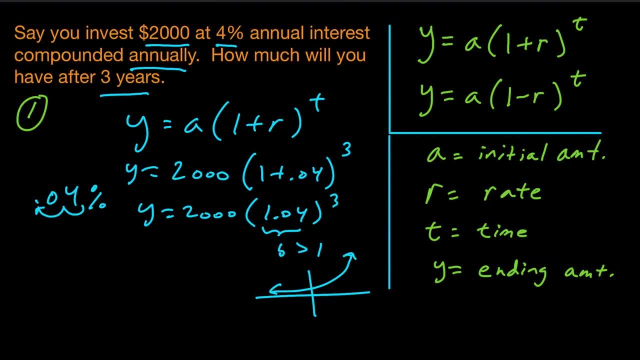 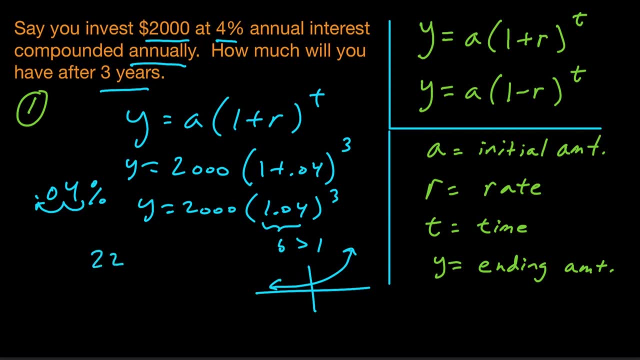 as time continues on. And now what we're going to do is we're going to put that into the calculator and see what our ending amount is. So do that real quick here. So I'm getting it's $2,249.73.. 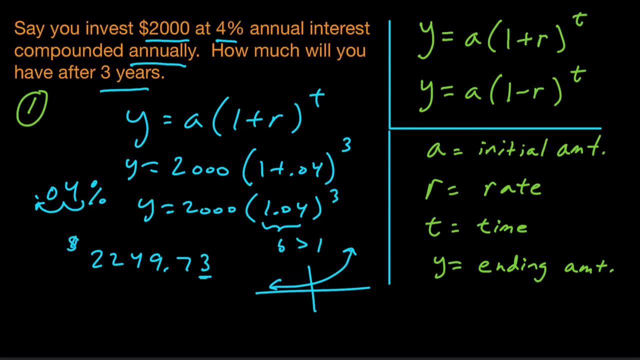 Be careful here. you want to always round to the two decimal places, to the pennies. So originally I got 0.728 and that eight. I rounded that two up to a three, So that's going to be your ending amount after three years. Okay, now for. 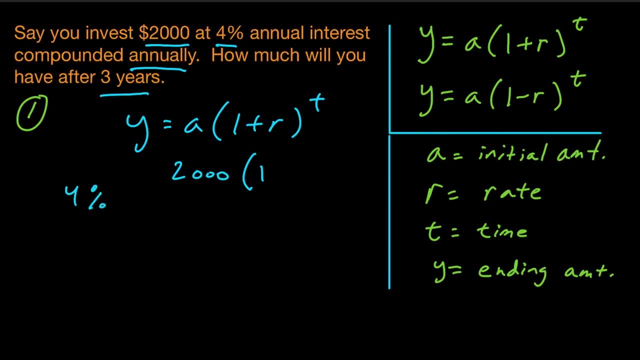 growth is 4%. Now, remember 4%. to convert that to a decimal, you move the decimal two places to the left, so that's going to end up being 0.04, and the time? that's, in this case, three years. So if we 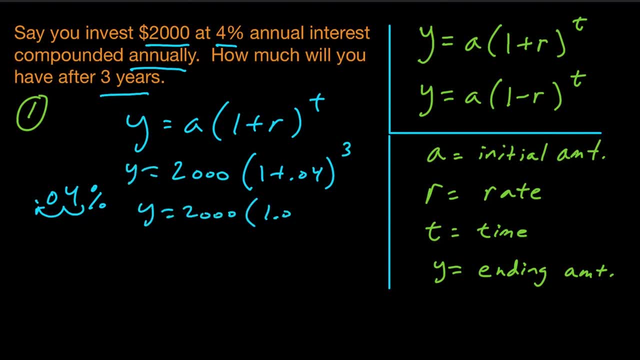 simplify a little bit. we get: y equals 2,000, 1.04 to the third. Notice: this base here is greater than one, which means that this is going to be an exponential growth function. It's going to grow, it's going to get larger and larger. 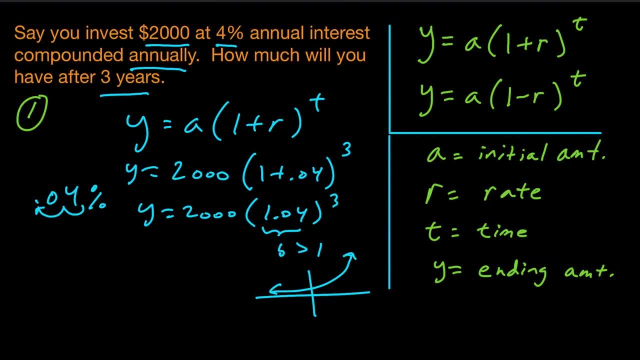 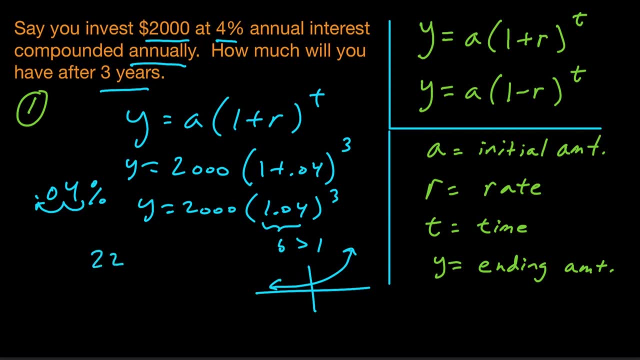 as time continues on. And now what we're going to do is we're going to put that into the calculator and see what our ending amount is. So do that real quick here. So I'm getting it's $2,249.73.. 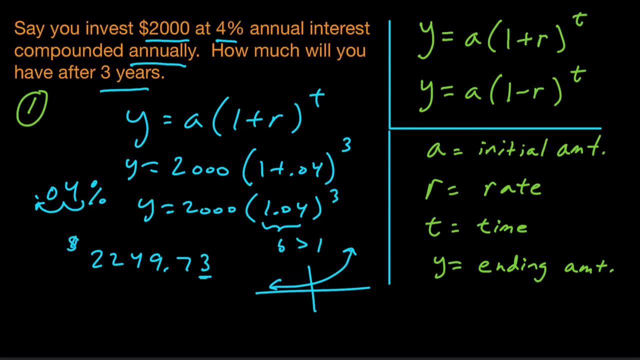 Be careful here. you want to always round to the two decimal places, to the pennies. So originally I got 0.728 and that eight. I rounded that two up to a three, So that's going to be your ending amount after three years. Okay, now for. 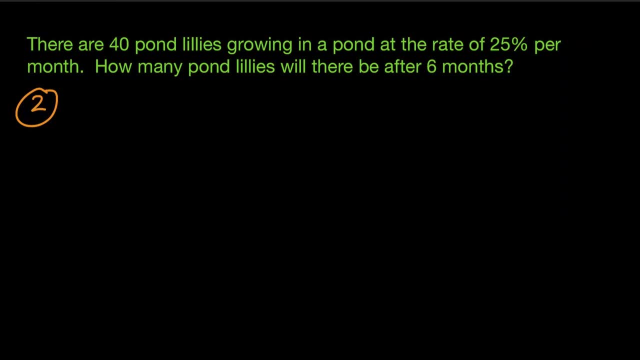 example two. let's try this one. So it says there are 40 pond lilies growing in a pond at the rate of 25% per month, And how many pond lilies will there be after six months? So again, this is an. 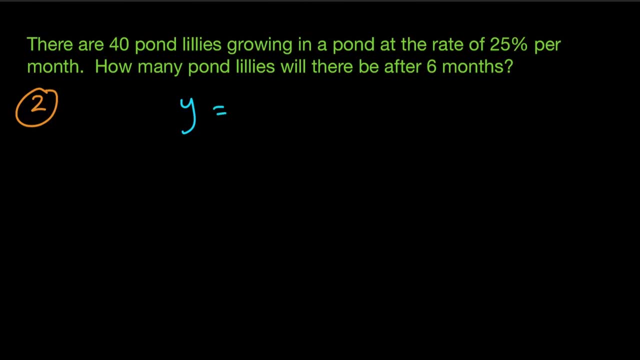 exponential growth function because it's obviously growing. the pond lilies are growing at a rate of 25% per month. So we're going to use that first equation: y equals a times one plus r to the t. Our starting amount is the 40 pond lilies and 25%. we're going to move that decimal two places to the left. 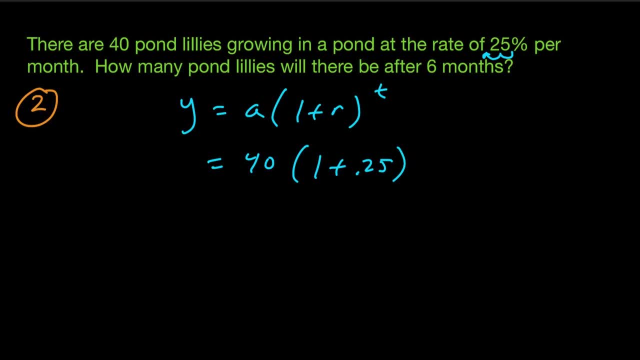 so that comes out to 0.25.. And we want to find out how many pond lilies there will be after six months. We're going to use six. Now in this problem everything was done in months. like the rate of growth was 25% per month. the time was months. So if we simplify this a little bit further, we get. 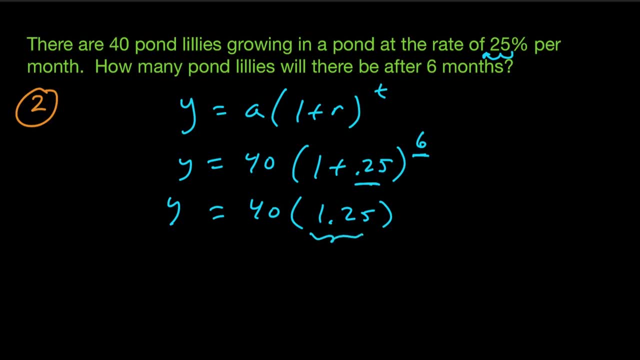 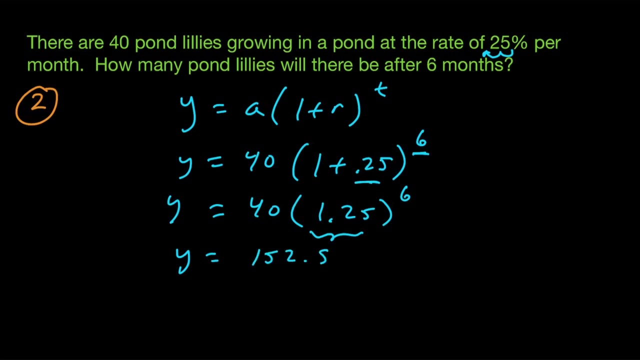 40.. Our base is 1.25.. That represents the growth factor, like what you're multiplying by each month And you're doing that six times And we're going to see how many total pond lilies there are after six months. So let's see what we get here. Go ahead and check my work. So I'm getting 152.59. 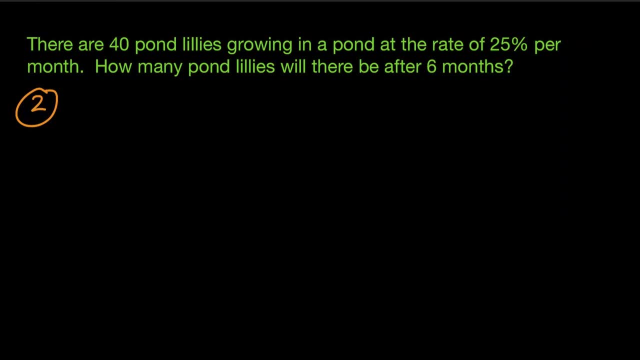 example two. let's try this one. So it says there are 40 pond lilies growing in a pond at the rate of 25% per month, And how many pond lilies will there be after six months? So again, this is an. 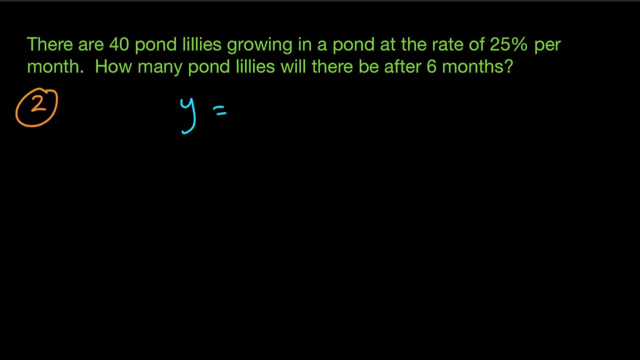 exponential growth function because it's obviously growing. the pond lilies are growing at a rate of 25%, So we're going to use that first equation: y equals a times one plus r to the t. Our starting amount is the 40 pond lilies And 25%. we're going to move that decimal two places to the left. So 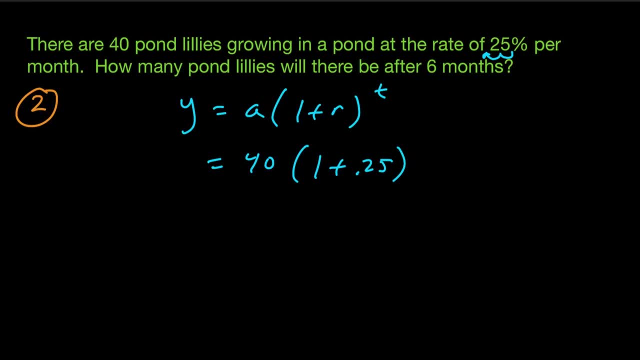 that comes out to 0.25.. And we want to find out how many pond lilies there will be after six months. we're going to use six. Now, in this problem everything was done in months. like the rate of growth was 25% per month. the time was months. So if we simplify this a little bit further, 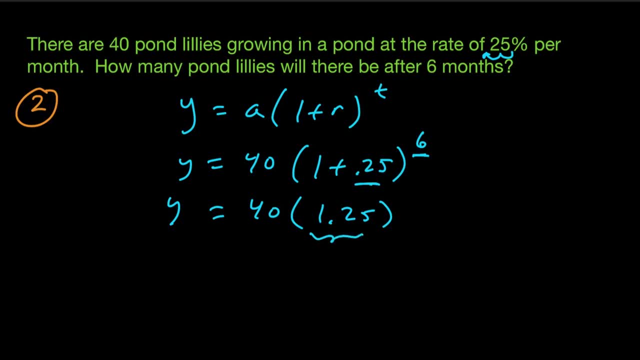 we'll get to about 40.. Our base is 1.25.. That represents the growth factor, like what you're multiplying by each month, And you're doing that six times And we're going to see how many total pond lilies there are after six months. So let's see what we get here. Go ahead and check my work. 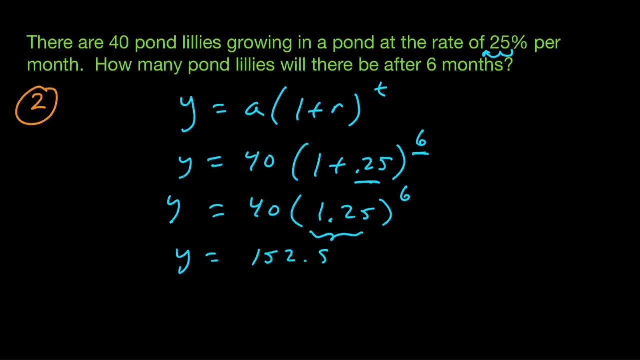 So I'm getting 152.59. But we're rounding to the nearest pond lily. So since this is 0.5, I'm going to round that up to 153, approximately 153 pond lilies, And you got it Okay. last problem here: See, if you can do this one on your own, We'll go through. 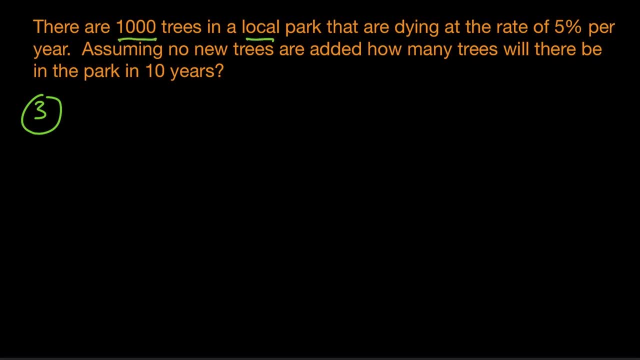 it together. But there are 1000 trees in a local park and they're dying at the rate of 5% per year. Okay, assuming no new trees are added to the park, how many trees will there be in 10 years? 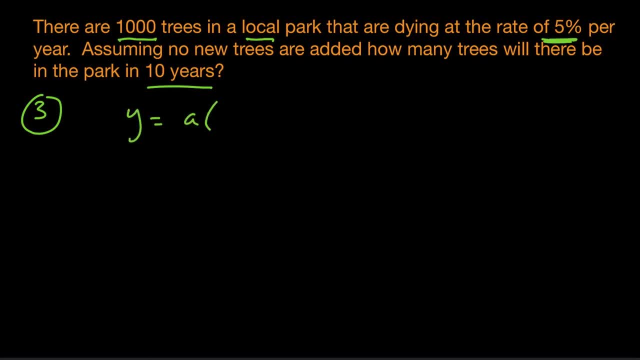 Okay, so this one we're looking at an exponential decay function, So it's going to look like this form here, where it's one minus r And you can see that our initial amount was 1.5.. So we're going to. 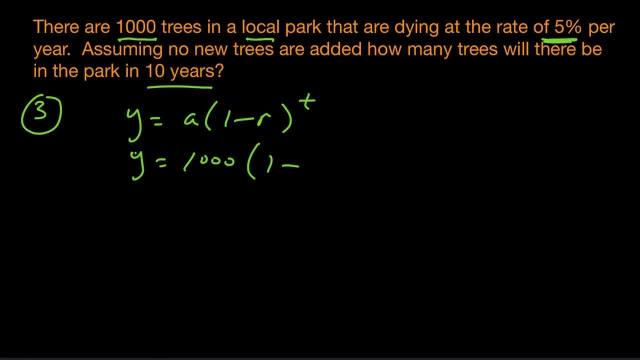 get 1000 trees. That's our a value And it's going down by 5% per year. Now remember, with 5% we're going to move that decimal point one to the left, So that's going to be put our placeholder in. 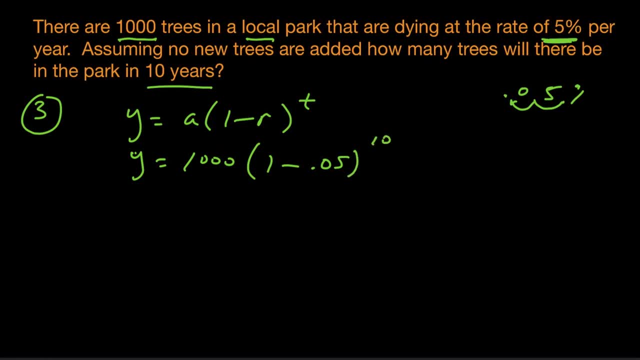 there 0.05.. And we don't know how many trees are after 10 years, So time is 10.. So if we simplify this a little bit here, we get 0.95.. And notice that 0.95 is less than one, which means that this: